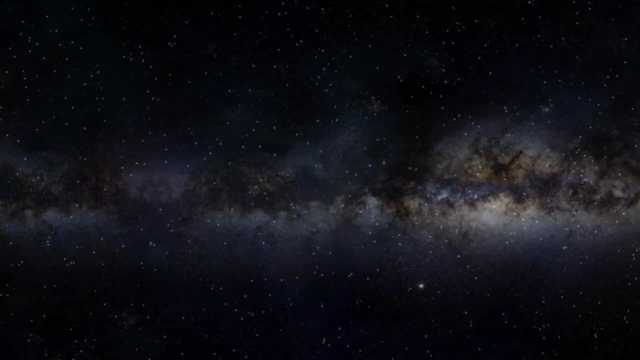 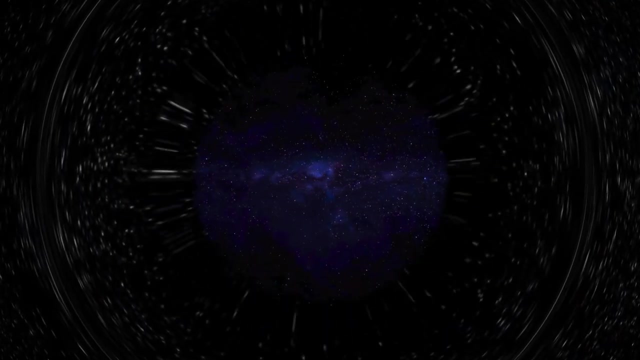 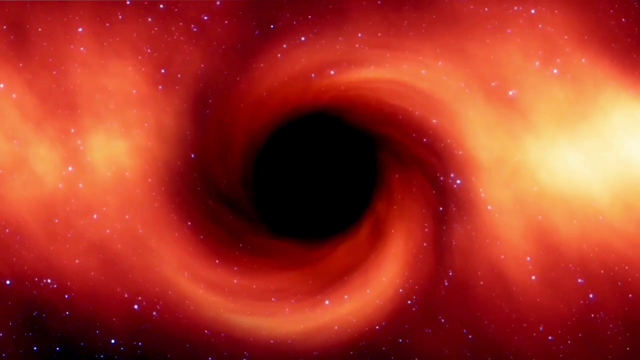 grow darker and darker with time. These dying stars will eventually turn into black holes and our universe will be dominated by these black holes. The black holes also will not survive for infinite time, as they emit Hawking radiation. A related scenario is the heat death According to. 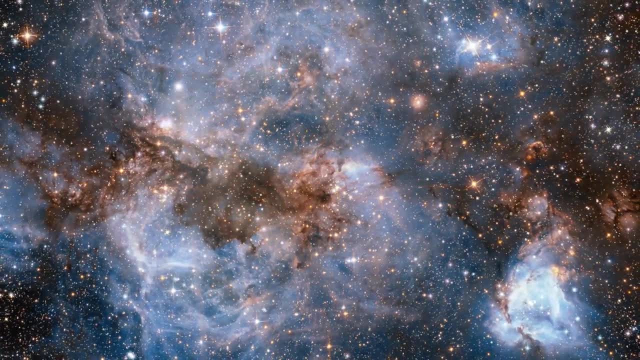 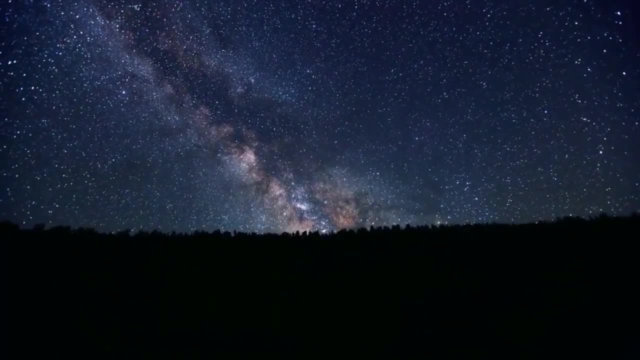 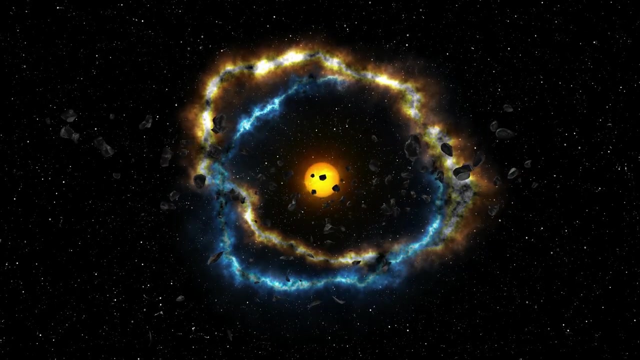 it, the universe goes to a state of maximum entropy in which everything is evenly distributed: There are no gradients, which are needed to sustain information processing, one form of which is the life Theory number 2. The Big Rip. According to the Big Rip theory, the universe 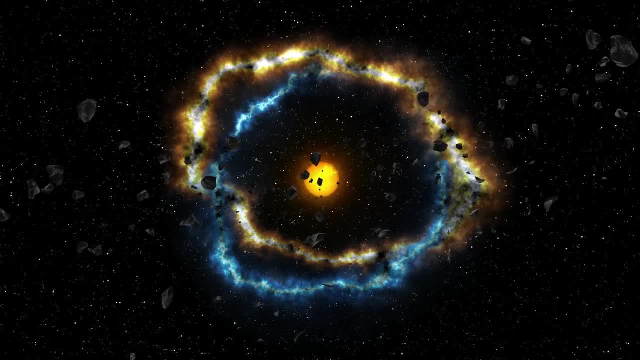 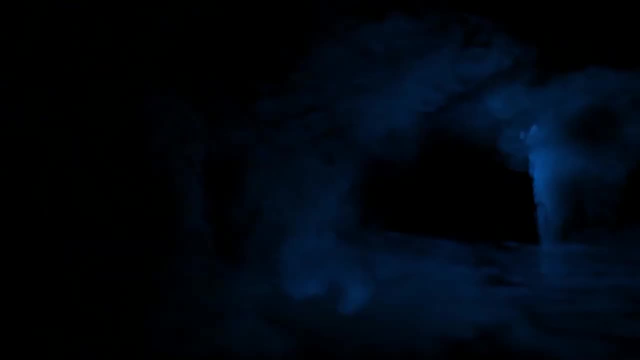 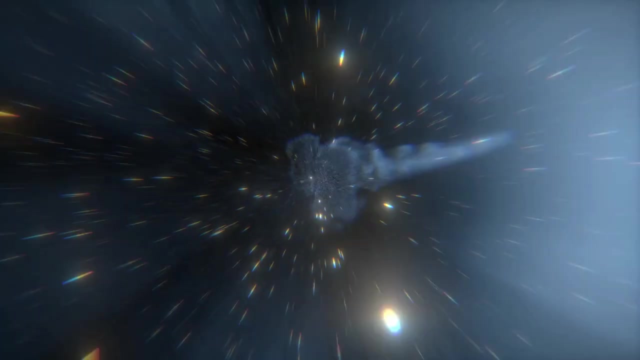 expands so fast that the gravitational force of attraction cannot compensate it and tears it apart. If the density of dark energy increases with time, it will cause the rate of acceleration of the universe to increase. It will lead to a steady increase in the Hubble constant. 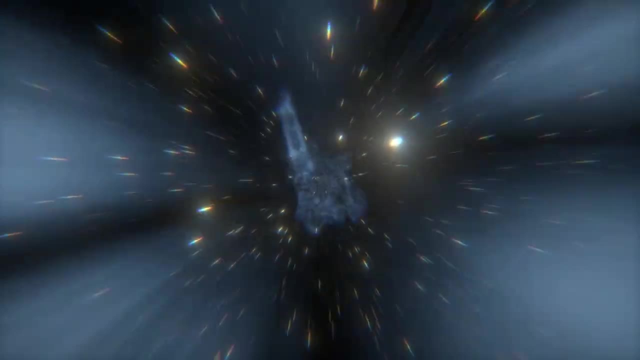 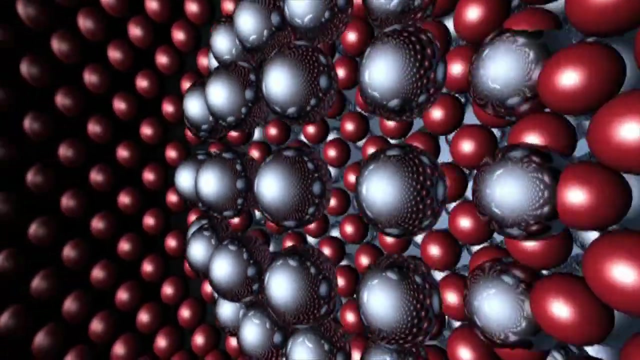 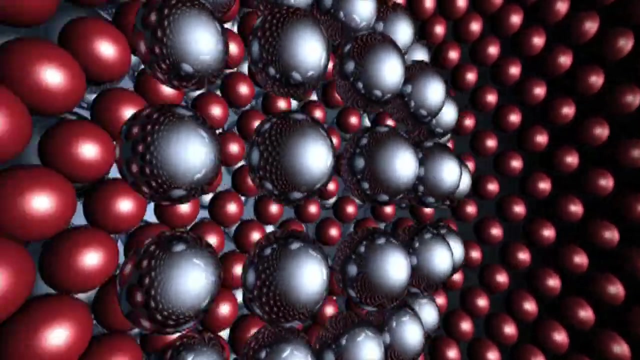 As a result, eventually, all the matter present in the universe will disintegrate into unbound elementary particles and radiation, As the dark energy density and the expansion rate of the universe becomes infinite. the end state of the universe will be a singularity. 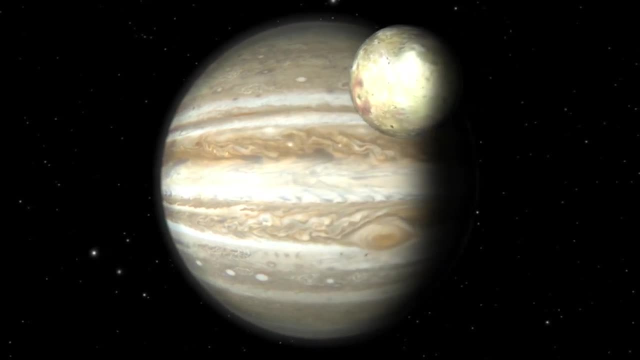 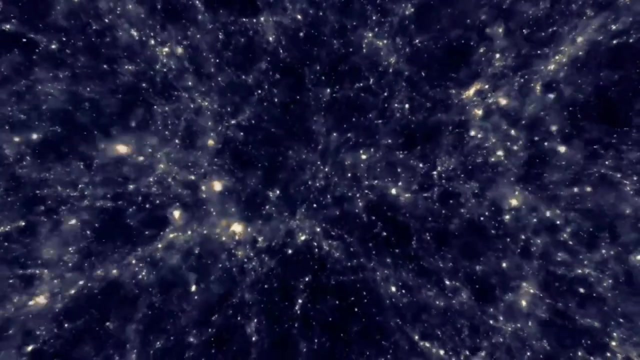 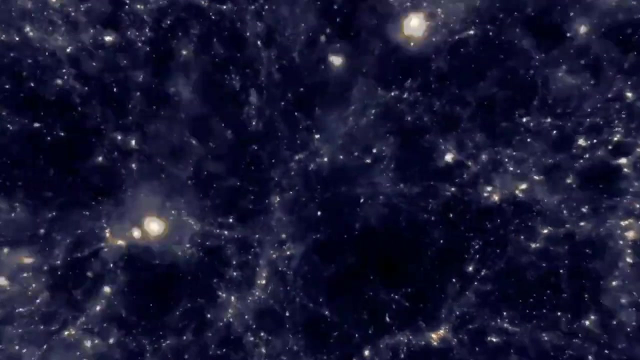 Theory number 3. The Big Crunch. The Big Crunch hypothesis states that the universe will not continue to expand forever. This theory assumes that the average density of the universe will be enough to stop its expansion and it will start to contract Because of this continued. 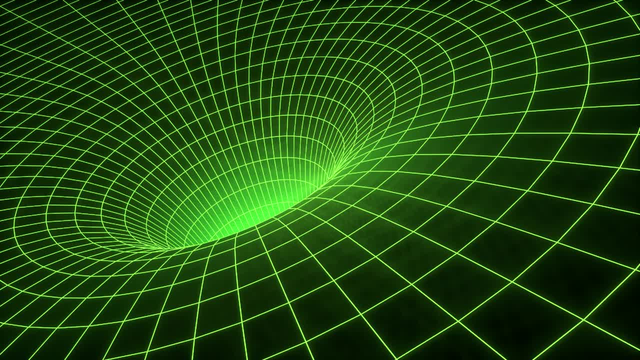 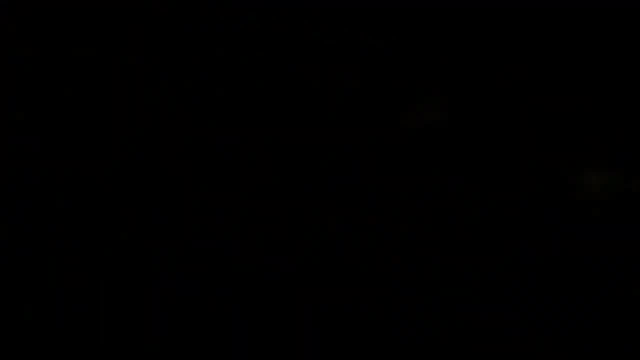 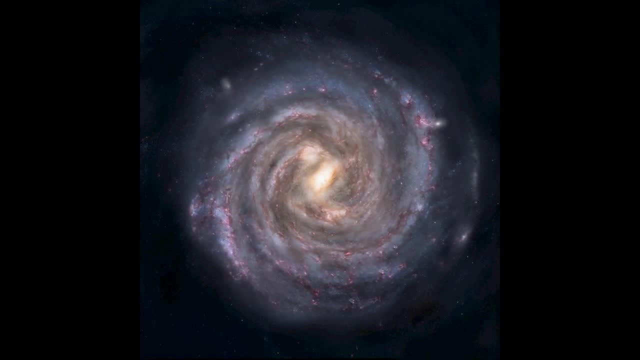 contraction, all the matter present in the universe will disappear. All the matter and space-time in the universe would collapse into a dimensionless singularity. This is the reason why it is named as the Big Crunch. At this stage, the universe will be at a point from where it started: the Big Bang. This scenario allows the Big Bang to.